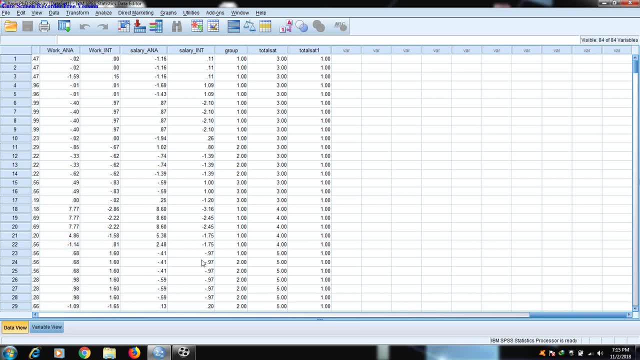 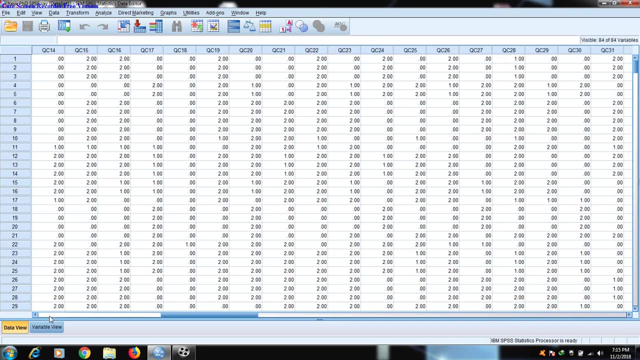 Hi, this is Dr Yasir Hayat Mughal and welcome to stats for everyone. Today we are going to learn about how to divide one variable into high, average and low categories or groups or levels. So in this case, we have seven items for job satisfaction. This is item 1, item 2,, item 3,, 4,, 5,, 6 and 7.. 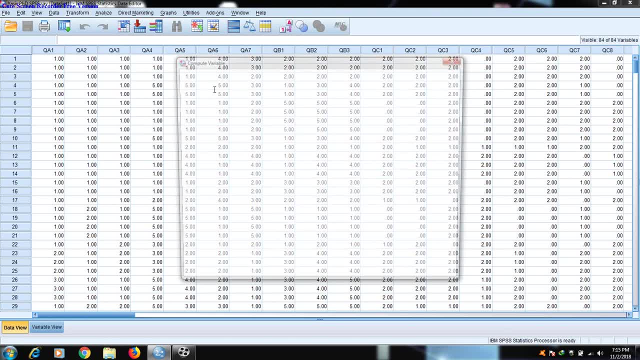 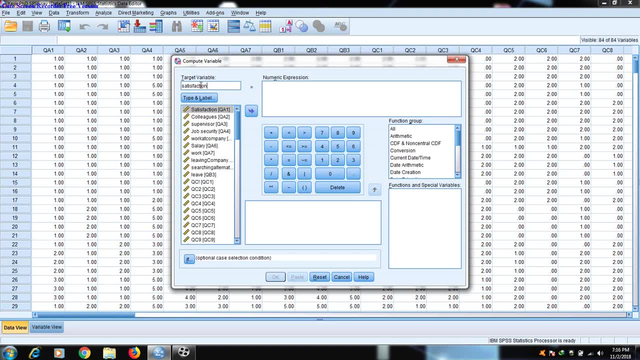 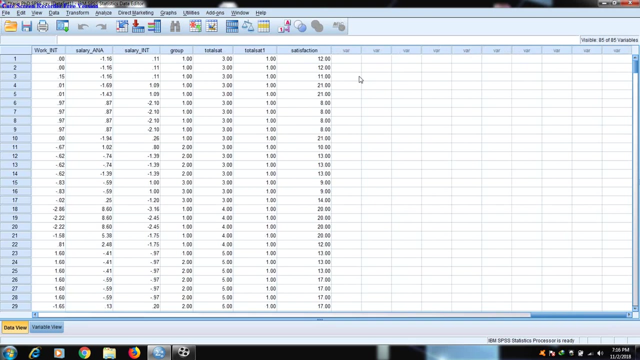 So first of all we have to transform and compute variable and we have to calculate this total satisfaction, and you have to bring all these variables into this box. So we have to click OK and at the end of this data view you can see that we have the new variable satisfaction. This is created. 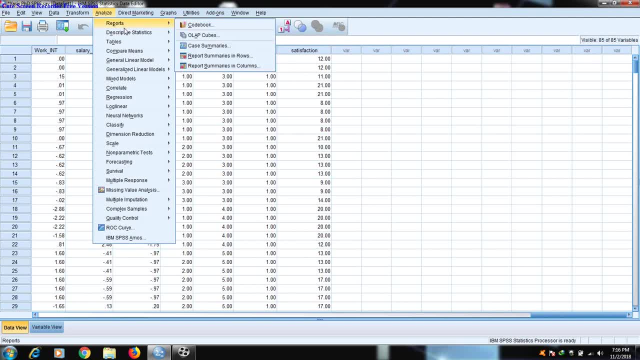 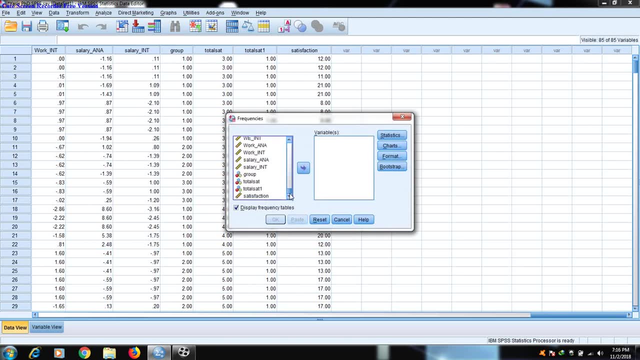 So first of all we have to go to analyze and we have to go to descriptive statistics and in descriptive we have to check the frequencies Of this new variable. So bring this satisfaction into variable box, This one, and make sure this is checked and click OK. 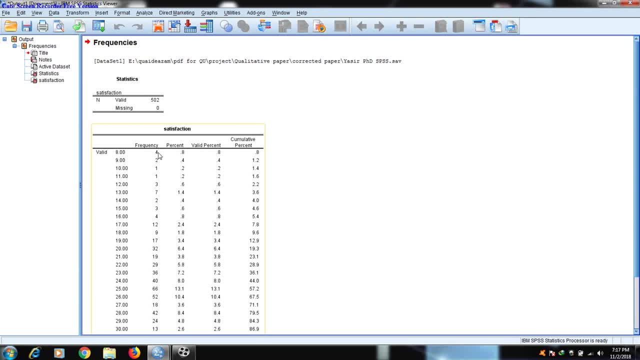 So here we can see that the lowest value is 8 and the highest value here we have is 35. So we have to check the median of this data. So we have to check the median of this data And we have to check the median into three stages. 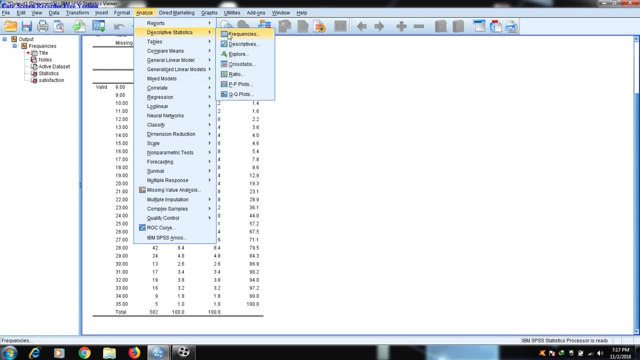 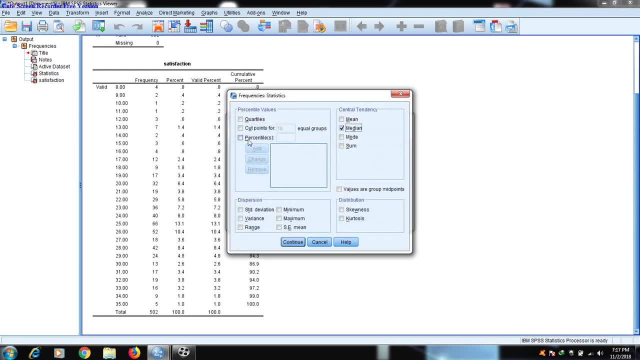 So first of all go to analyze again descriptive statistics, frequencies, and you have to click on the statistics, Click on median and here you can see the percentile If you divide 100 into three categories. so we have: first is 33 add and the second is 66 add and the third is 100. 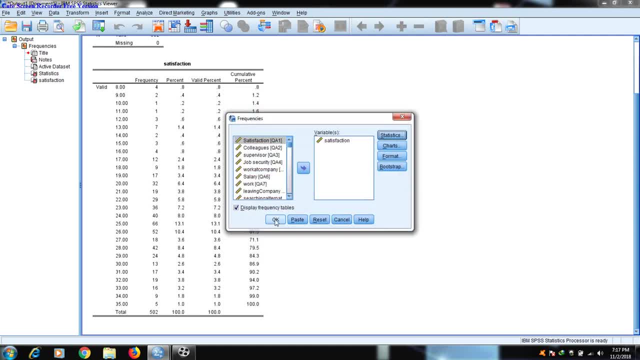 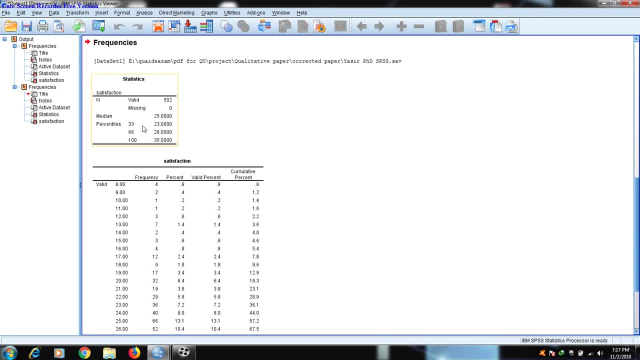 And at OK. So you have to click continue and OK. So here you can see that we have first median at 33, which is at 23, the second 66 percent is at 26 and the hundred is at 35. So we have to now record. 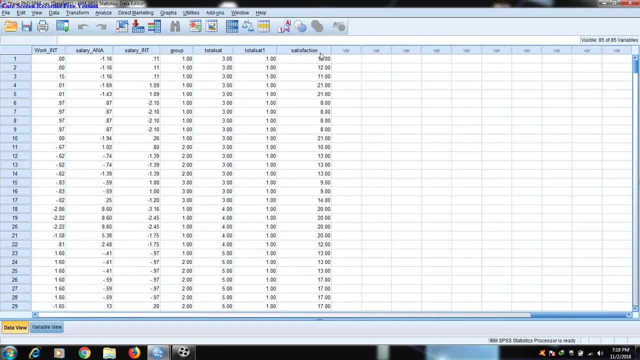 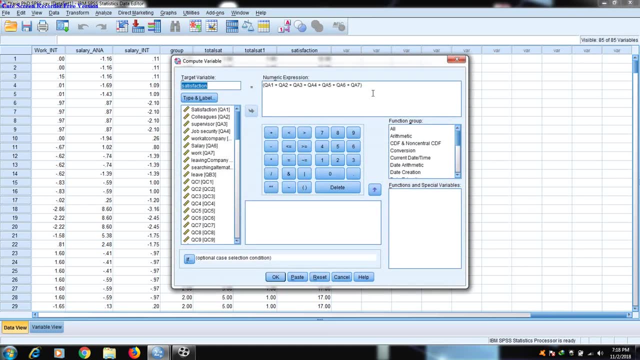 We have to create a variable, just same variable of satisfaction. We have to copy, we have to copy and paste here. so go to transform, click on compute variable and click here. clear is and you have to rename each satisfaction one and you have to bring this satisfaction here. 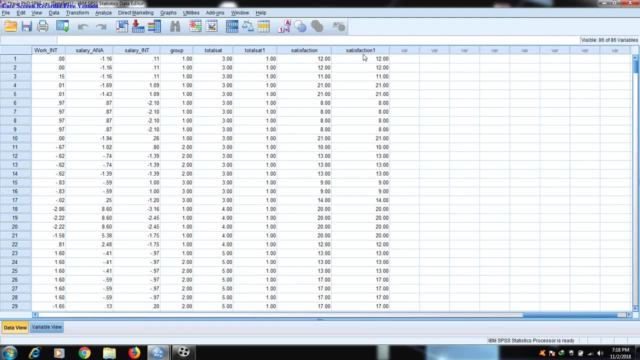 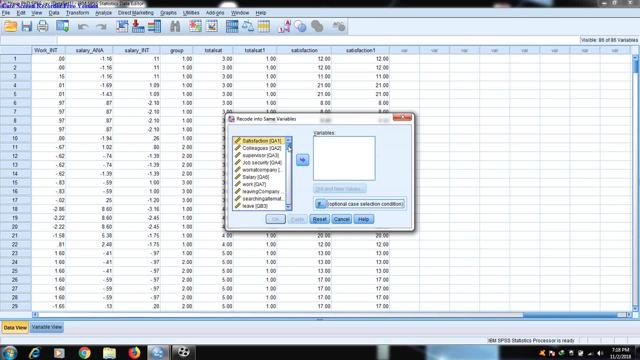 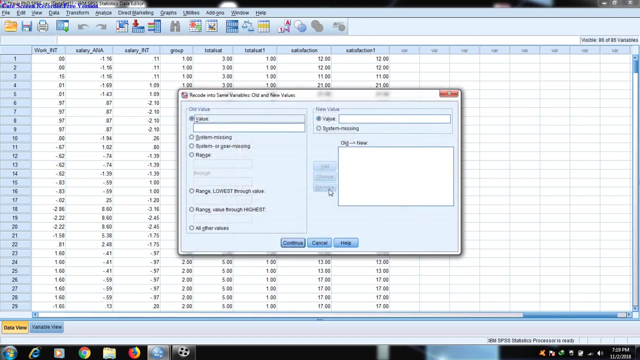 and click ok, so we have the same variable. you can see 12, 12, 11, 21. so first of all you have to go to transform again and click on record into same variable. so okay, bring the new variable into the variable box, satisfaction 1, and click here on old. 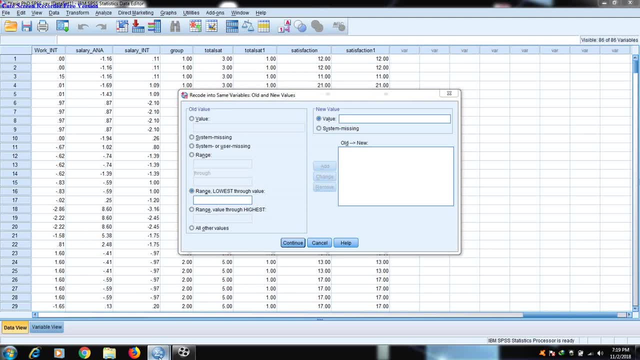 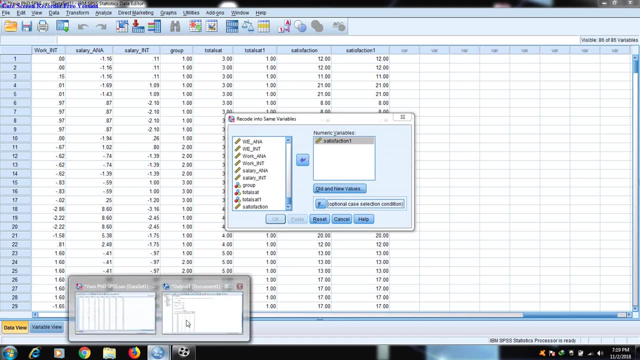 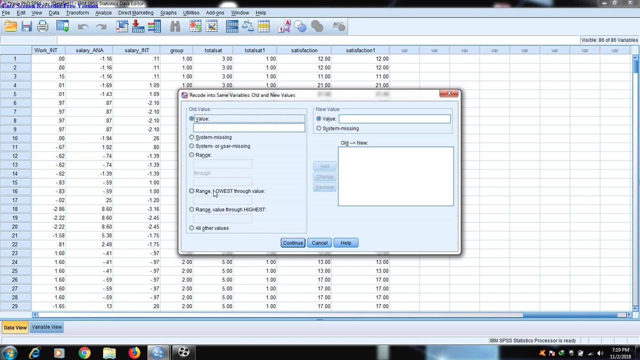 and new values. here you have the lowest value, if you remember the lowest value we have. the lowest value we have is 23. okay, so we have to add here the lowest value, 23, and we call it a group 1 and add here. so the second value we have is 26. okay, so here. 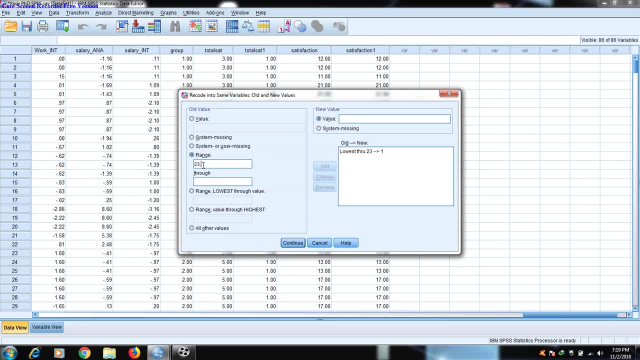 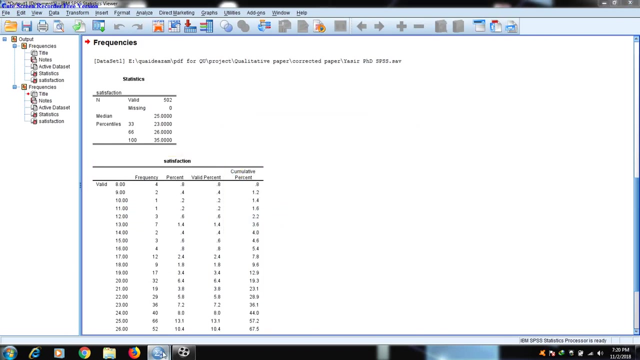 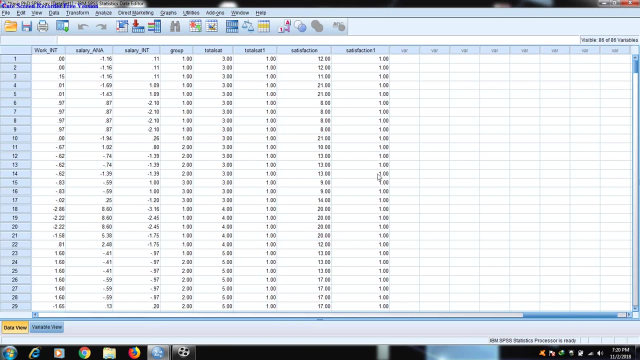 we have to give a range 23, 0.00001 to 26, okay, and we call it group 2 and 8, and here, from 26.000001 to 35, we call it group 3 and 8, and click continue and click OK. you can see here all this is converted into new variable. so we: